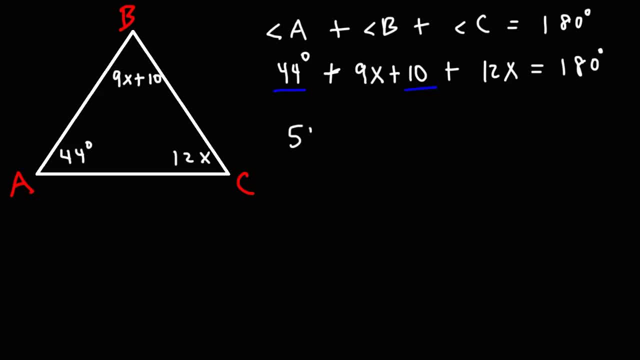 So we're going to add 44 plus 10. So that's going to be 54. 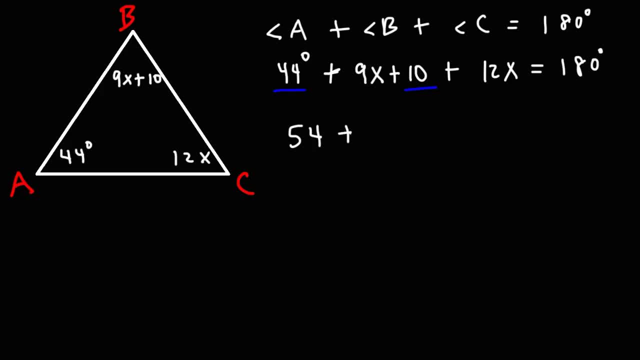 We don't have to worry about the degree symbol for now. And then 9X plus 12X, that's 21X. And that's going to equal 180. 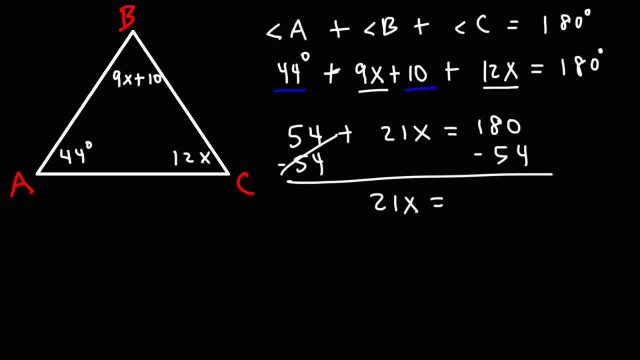 So now let's subtract 180 by 54. 180 minus 50. Is 130. And 130 minus 4. 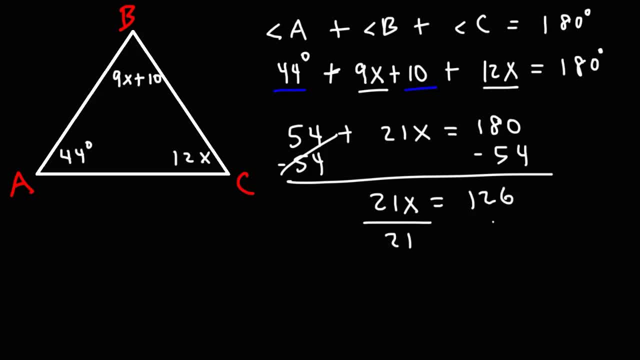 Is 126. Next we need to divide both sides by 21. 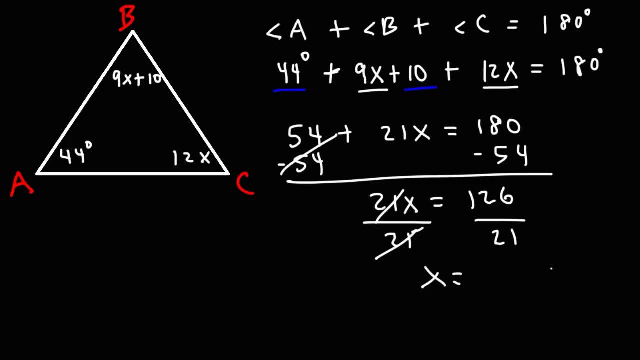 12 divided by 2 is 6. And 6 divided by 1 is 6. So 126 divided by 21 is 6. 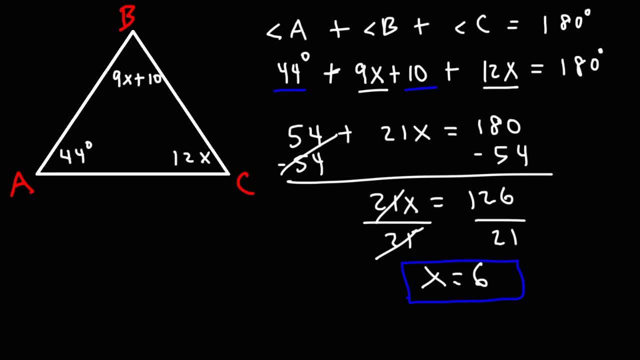 So now that we have the value of X. We can now determine the measures of angles B and C. So let's start with angle B. That's 9X plus 10. 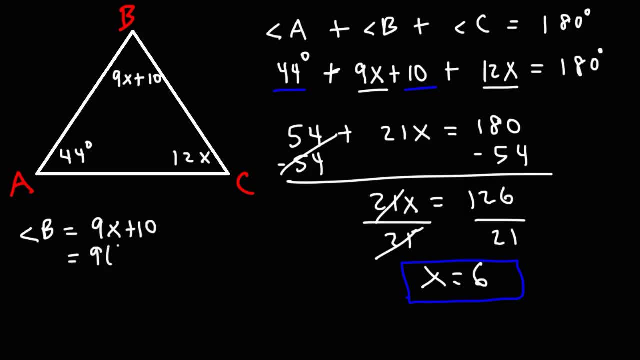 So let's replace X with 6. 9 times 6 is 54. Plus 10, that's 64. So angle B has a measure of 64 degrees. 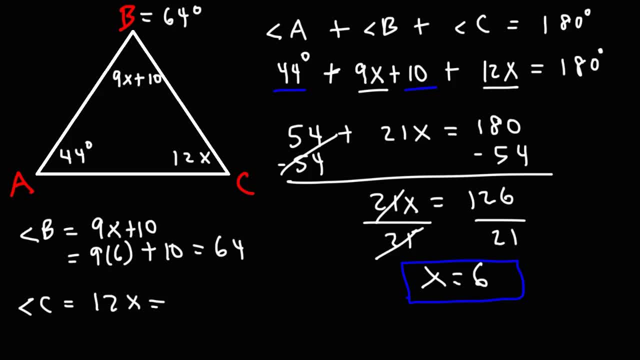 Now let's do the same thing for angle C. Which is 12X. If we replace X with 6, we'll have 12 times 6, which is 72. 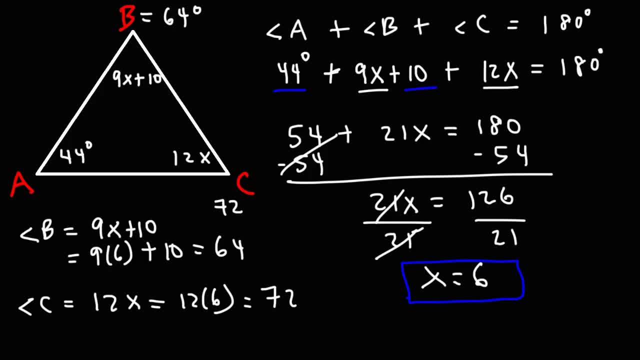 Now to check the work, to make sure that we have the right answers. We're going to use these three angles. 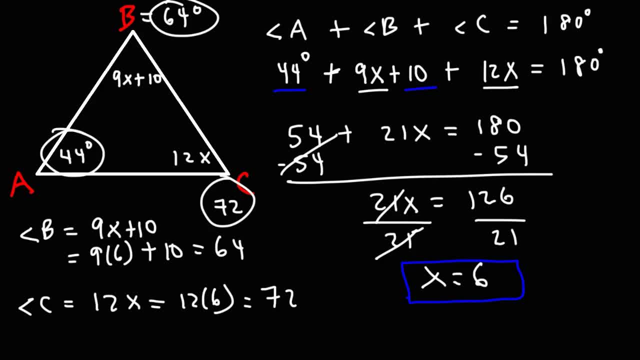 Must add up to 180. 44 plus 64 plus 72 is indeed 180. 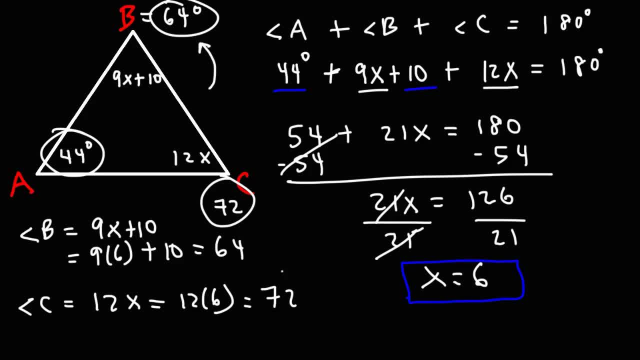 So that's how we could find the missing angles in this example problem. So B is 64. C is 72. 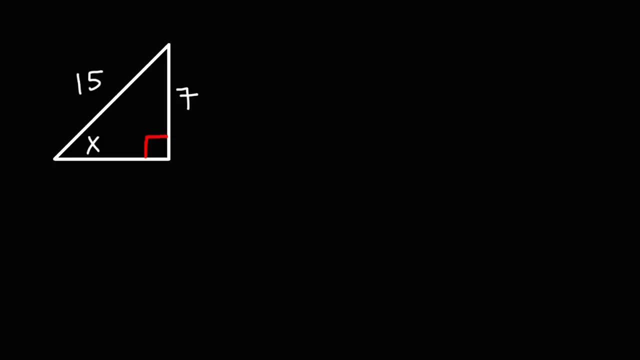 Now let's move on to our next problem. So in this problem, we have a right triangle. We have two sides of the right triangle. And we need to calculate the angle X. 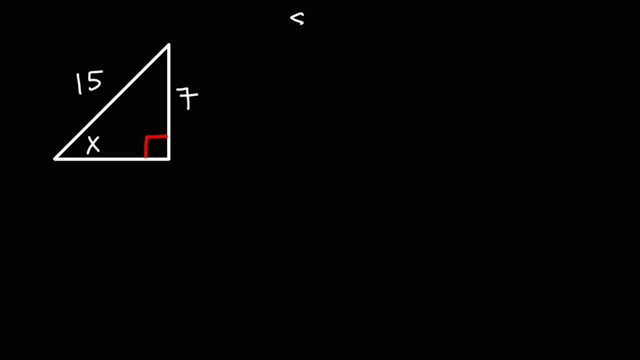 How can we do this? Well, there's something called SOHCAHTOA. 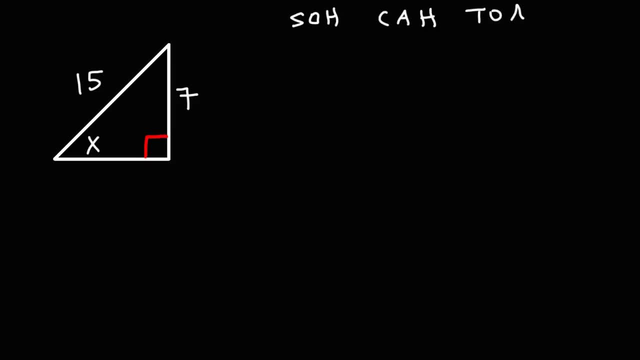 That will help us to get the answer. The SOH part in SOHCAHTOA tells us that sine of the angle that we're considering, that is angle X, is equal to the side opposite to angle X divided by the hypotenuse. 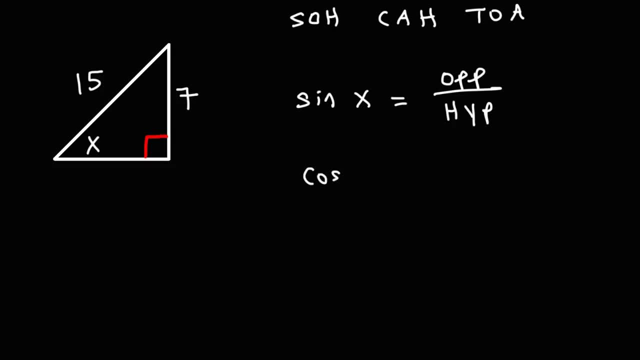 The CAH part in SOHCAHTOA tells us that cosine X is equal to, think of the letter A, is equal to the adjacent side relative to, to X, divided by H, the hypotenuse. 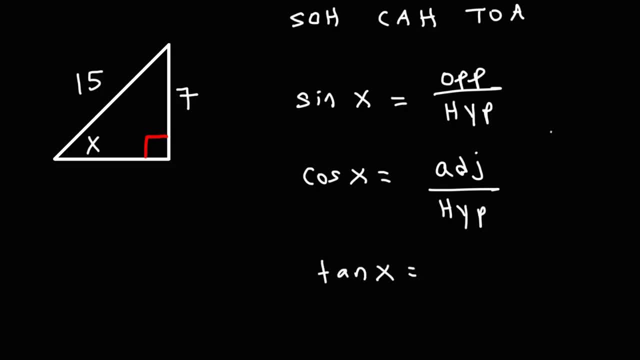 And then the last trig ratio, tangent. Think of TOA, O-A. So tan X is equal to the opposite side divided by the adjacent side. So we already know what the hypotenuse is. 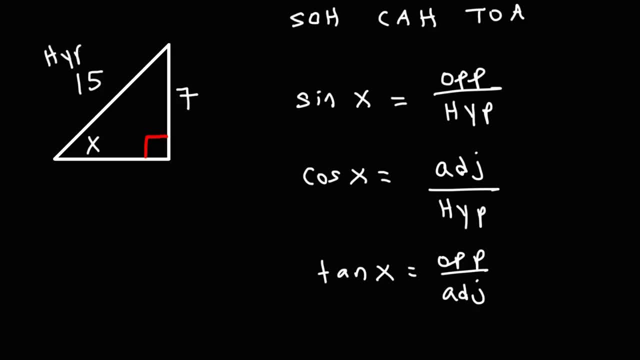 The hypotenuse is 15. It's always across the 90 degree right angle. It's always the longest side of, of the three sides in the right triangle. Opposite to X is 7. 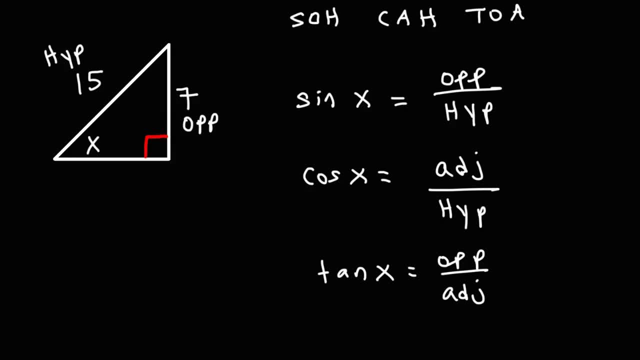 Adjacent to X, or right next to it, is that side. So notice that we only have two of the three sides of the right triangle. We have the hypotenuse and the opposite side. Therefore, which of the three trigonometric ratios should we use? Should we use sine, cosine, or tangent? Well, we have to use sine because we have the two sides that corresponds to this particular trig ratio. 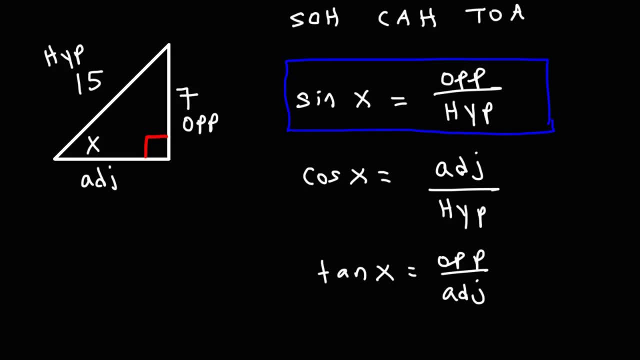 We have the opposite side and the hypotenuse. We don't have the adjacent side, so we can't use tangent, nor can we use cosine. 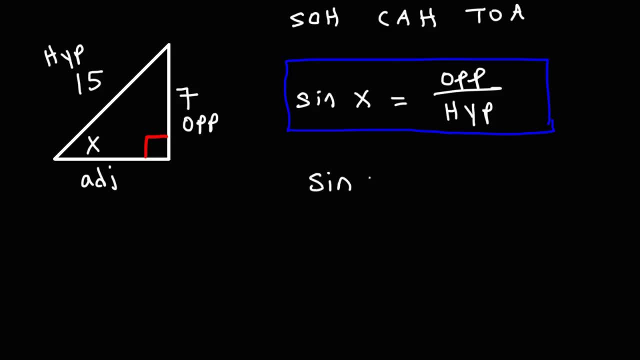 Now, let's go ahead and finish this problem. So we have sine X is equal to the opposite side, which is 7, divided by the hypotenuse, which is 15. 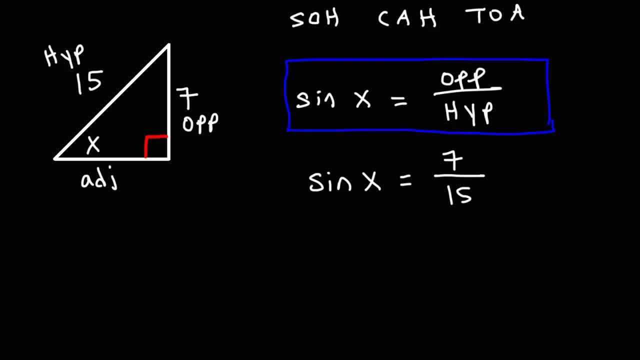 Now, in order to calculate X, we need to take the arcsine. 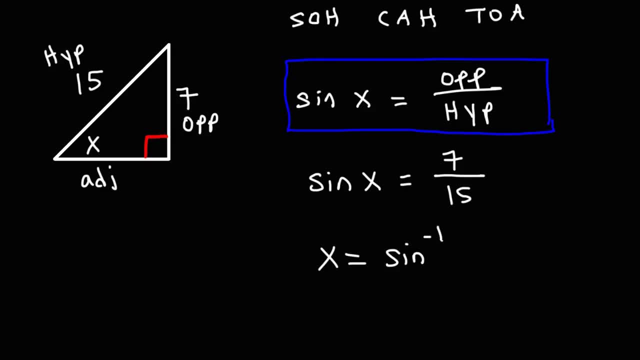 It turns out that X is equal to the arcsine of 7 over 15, or the inverse sine of 7 over 15. So you'll need your calculator for this. 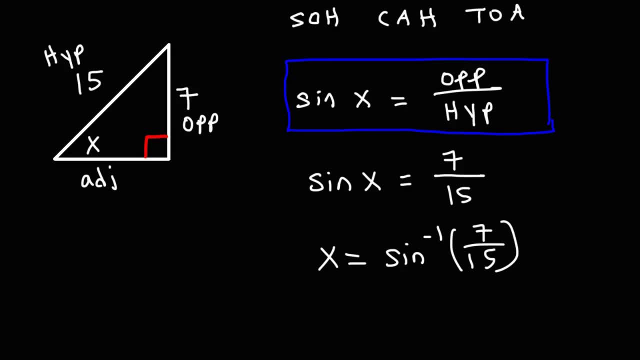 Make sure it's in degree mode, not in radian mode. If you type in arcsine or inverse sine 7 over 15, you should get this answer. 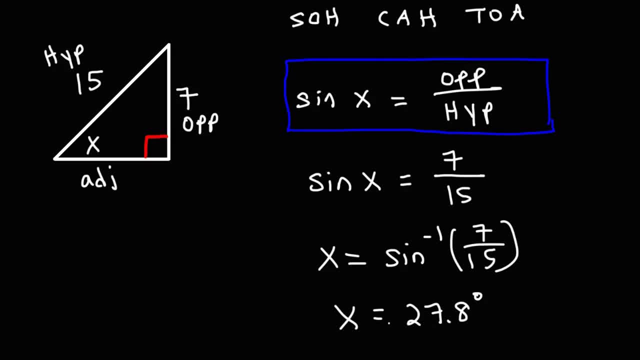 X is equal to 27.8 degrees. So this is the answer for this problem. That's how you can calculate the missing angle of a right triangle. 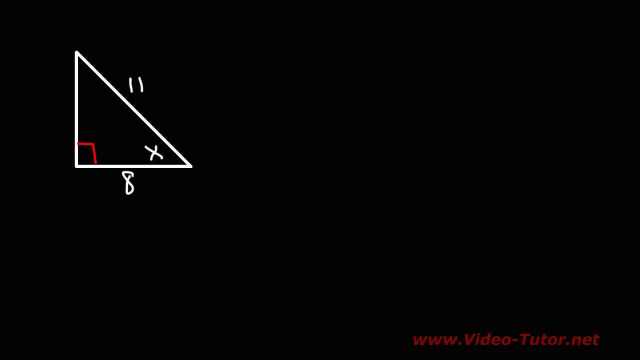 Here is another example that is similar to the last problem. Go ahead and calculate the value of X. So first, we need to determine which of the three trigonometric ratios we need to use. Across the right angle, we have 11. So that is the hypotenuse. And next to or adjacent to X, we have 8. So we know the adjacent side and the hypotenuse. So which of the three trigonometric ratios should we use? Sine, cosine, or tangent? Well, we need to use cosine because cosine is equal to the adjacent side over the hypotenuse. 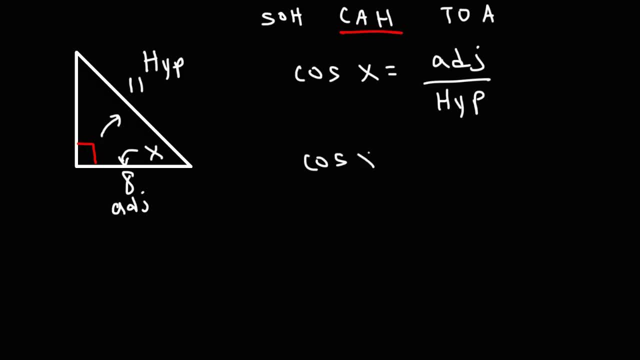 And we have both of those two sides. So the adjacent side is 8, the hypotenuse is 11. 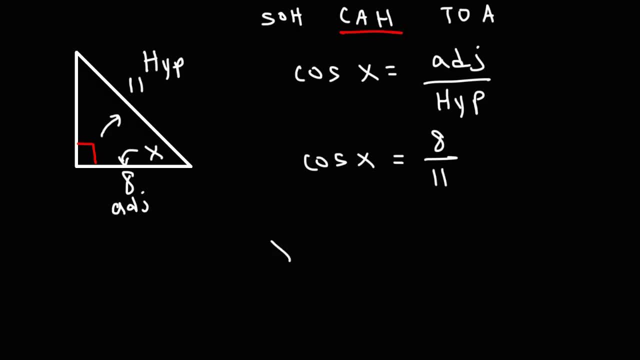 So if cosine X is equal to 8 over 11, then X is equal to arc cosine, or inverse cosine, 8 over 11. 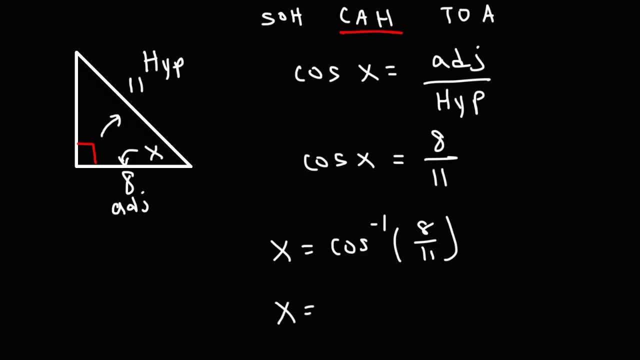 And using a calculator, you'll find that X is equal to 43.3 degrees. 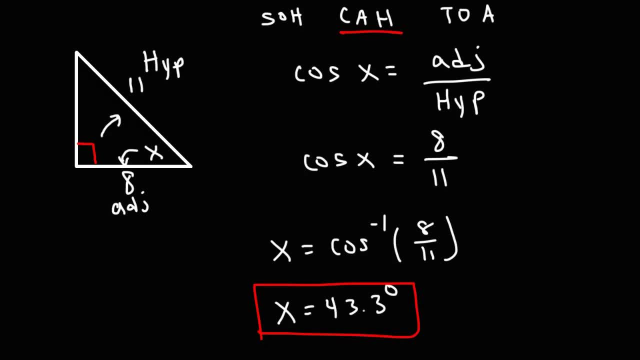 So now you know how to find the missing angle, or at least you know how to calculate the missing angle of a right triangle. Now let's try this problem. 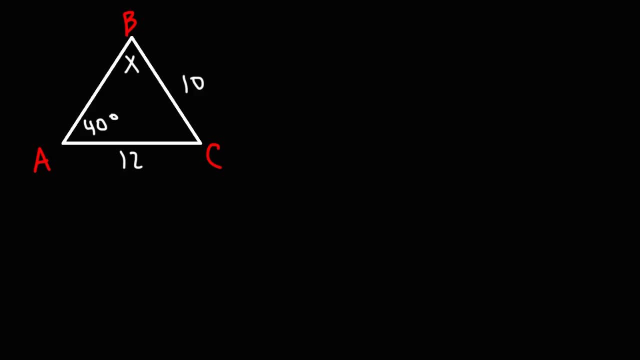 What is the measure of angle B? Or what is the value of X in this problem? 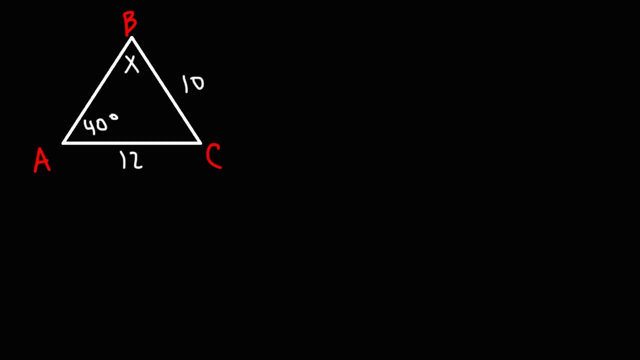 We don't have a right triangle, so we can't really use Sohcahtoa. That's not going to help us here. 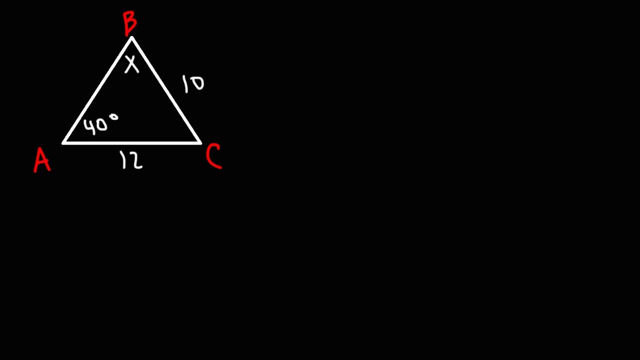 We don't have two of the three angles, so we can't use the fact that the three angles must add up to 180. 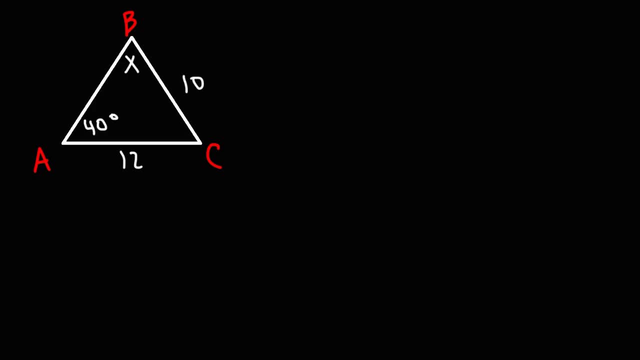 In this case, what we need to use is something called the law of sines. Sine of angle A over A is equal to sine of angle B. 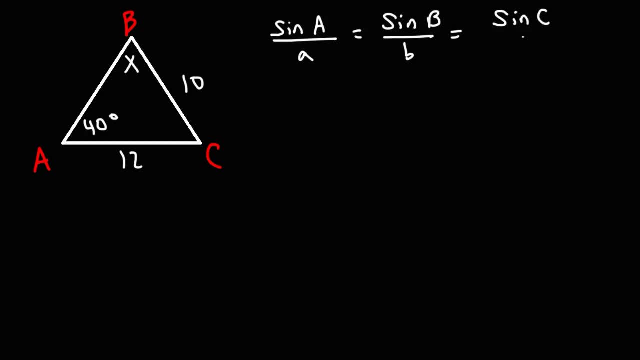 Over B, and that's equal to sine of angle C over C. So we know the measure of angle A, that's 40. 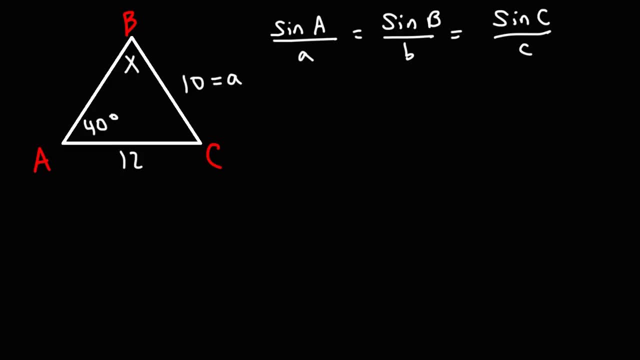 Across capital A, or angle A, is side A. So lowercase a is 10. 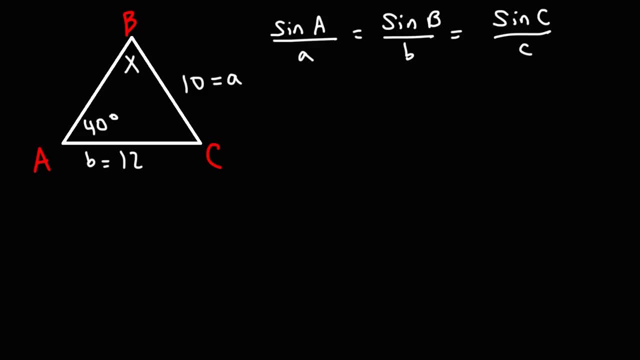 We know side B is 12, and we're trying to calculate angle B. So we only need these two of the three fractions in the law of sines. 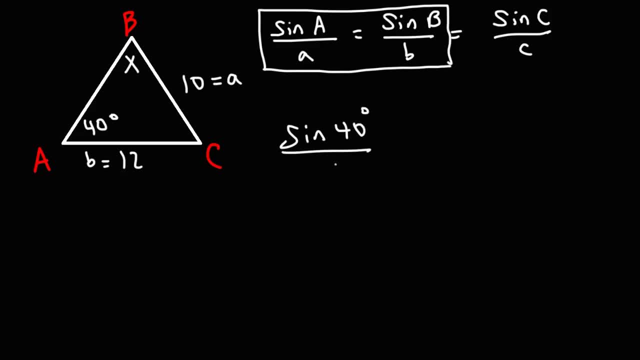 So let's replace angle A with 40. Side A is 10. 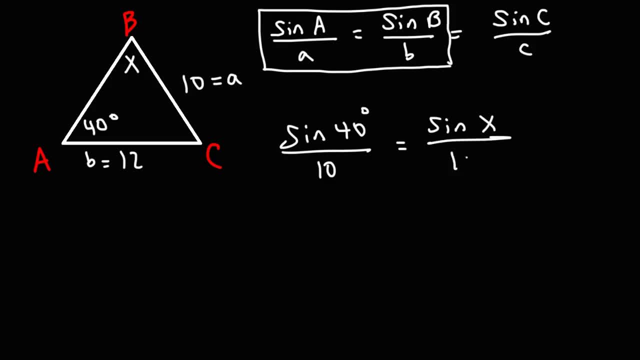 Let's replace capital B with X, and side B is 12. 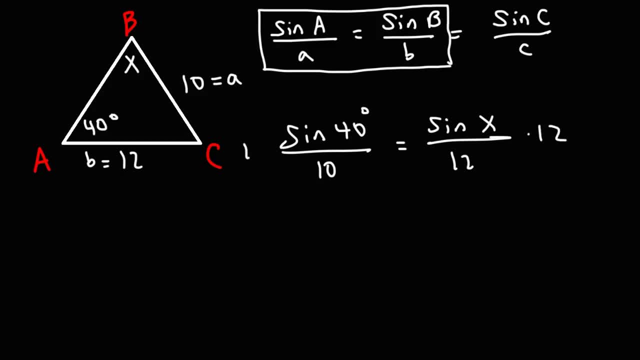 So what I'm going to do now is I'm going to multiply both sides by 12 to get rid of the 12 on that side. 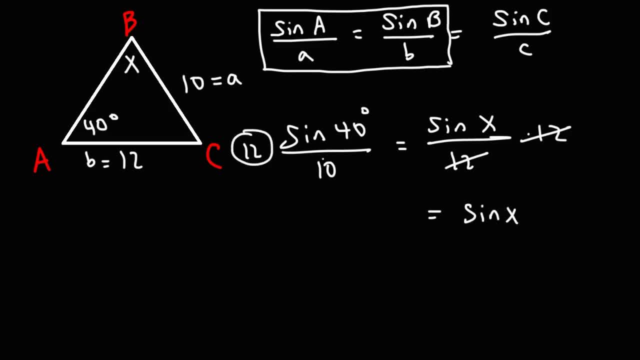 So I have sine X is equal to 12 divided by 10, which is 1.2 times sine of 40 degrees. 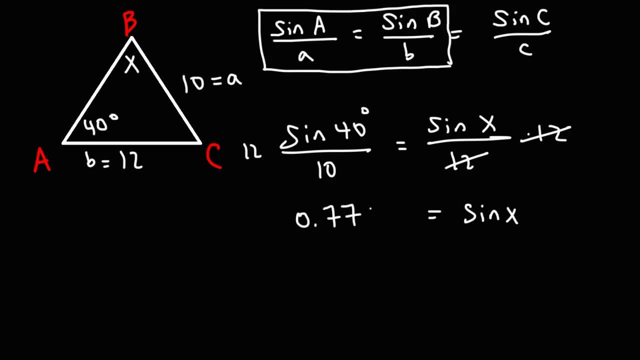 So this is equal to 0.77. 1, 3, 4, 5. 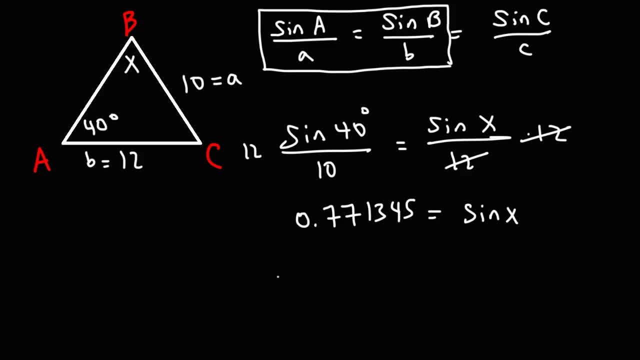 So if sine X is equal to this number, then X is equal to the arcsine of 0.771345. 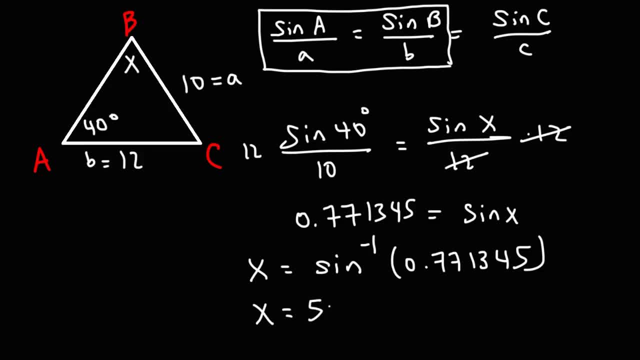 So if you plug this in, you should get 50.47 degrees. 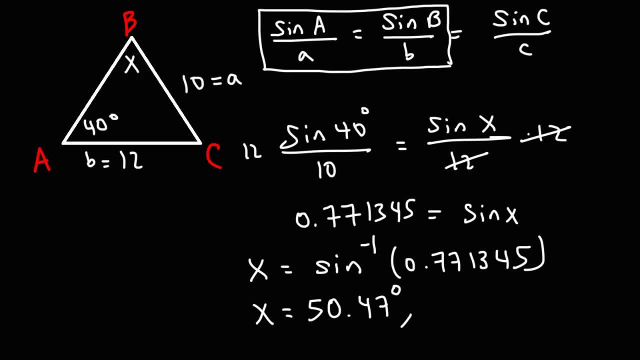 But this is not the only answer. The second answer, you get two possible answers. 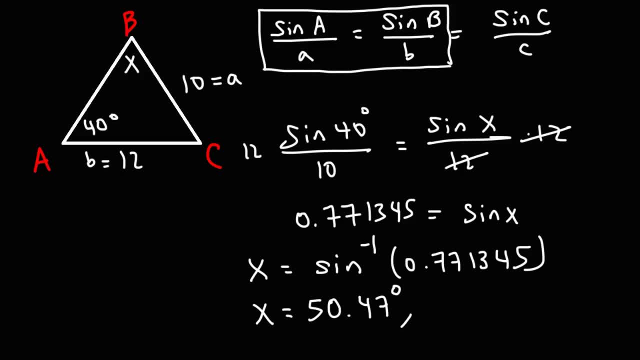 The second answer is 180 minus the answer that you just got, which is 129.53 degrees. 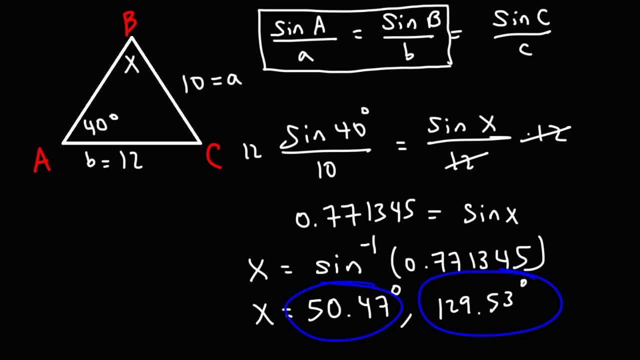 So you can potentially get up to two answers. Now the second answer, it may or may not be correct. 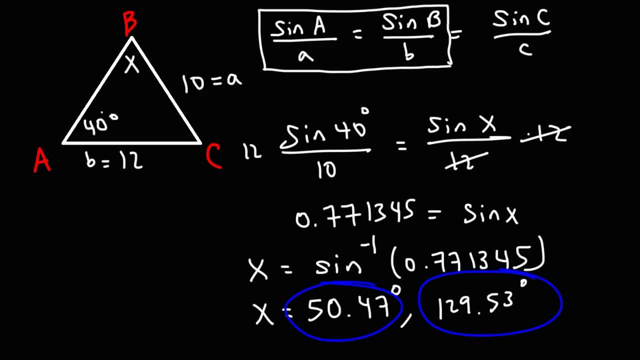 You have to check. And here's how you can check. Look at angle A and angle B. 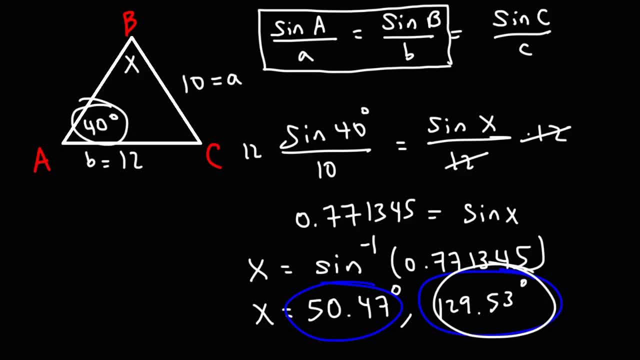 If these two angles add up to more than 180, then you know it's not possible. 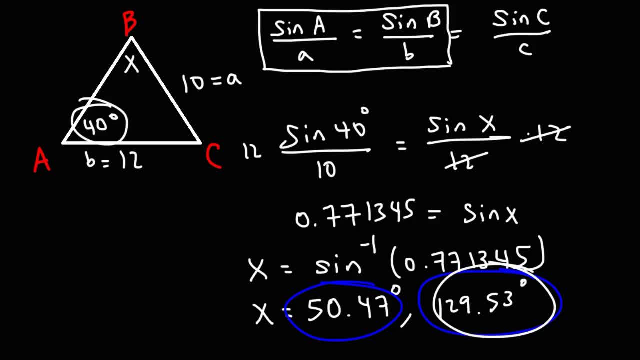 However, in this example, the sum total of those two angles is 169.53 degrees. 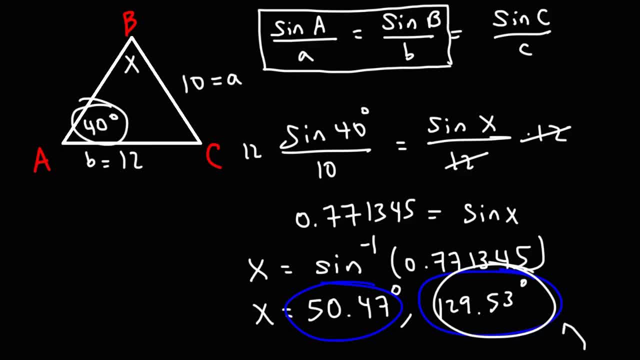 So it's possible to create a second triangle with this angle as angle B. 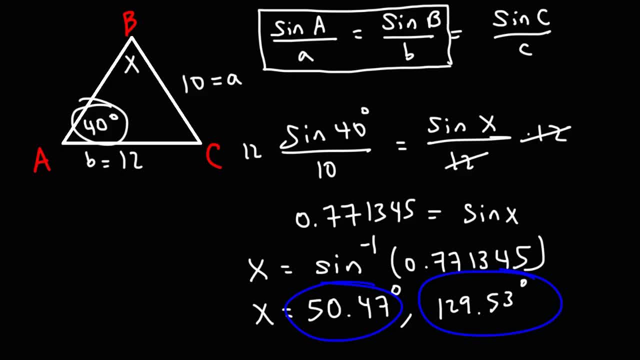 So therefore, we have two possible answers for angle B. Angle B can be equal to 50.47 degrees, or in the second, or in the second triangle, it can be equal to 129.53 degrees. 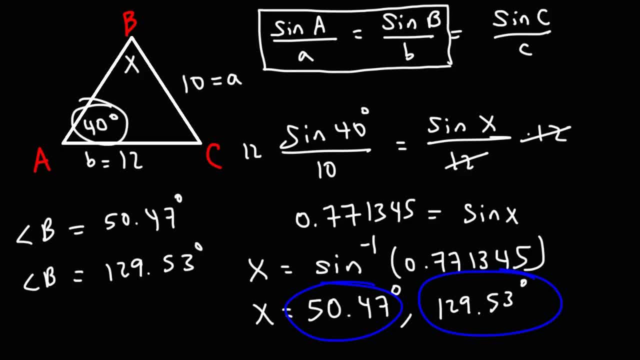 So whenever you're calculating the missing angle using the law of sines, just keep in mind that you can get two possible answers. 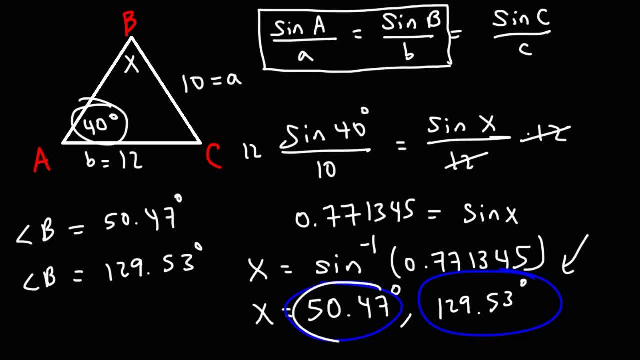 And remember, to get the second angle, it's simply 180 minus the first angle. 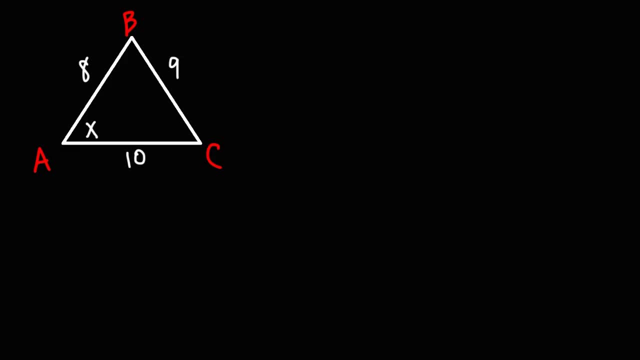 Now let's move on to our final example, where we know the three sides of a triangle, 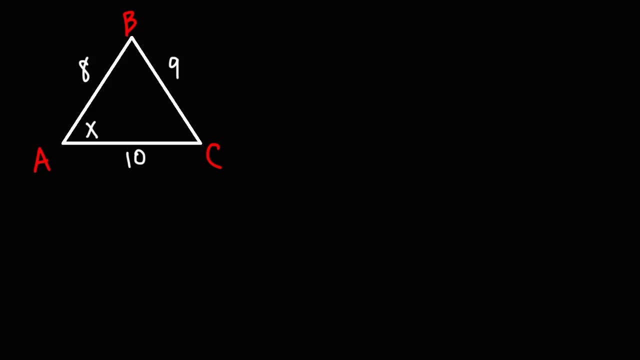 and we wish to calculate one angle inside that triangle. In this case, we could use law of cosines. 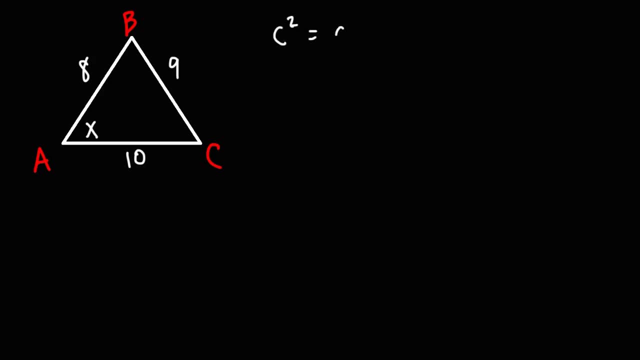 This is one version of the law of cosines. C squared is equal to A squared plus B squared minus 2AB times cosine of capital C, 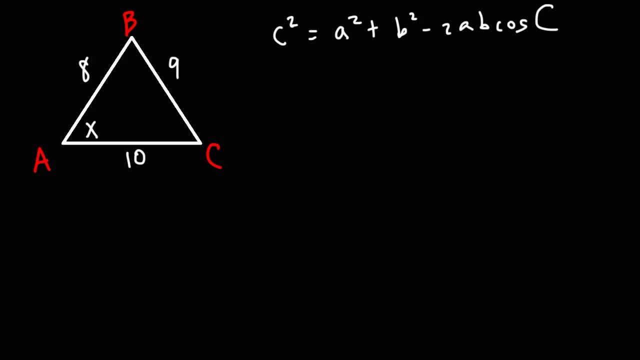 where capital C is angle C. Now we wish to calculate angle A, or capital A. So we're going to rearrange this equation, replace in C with A. 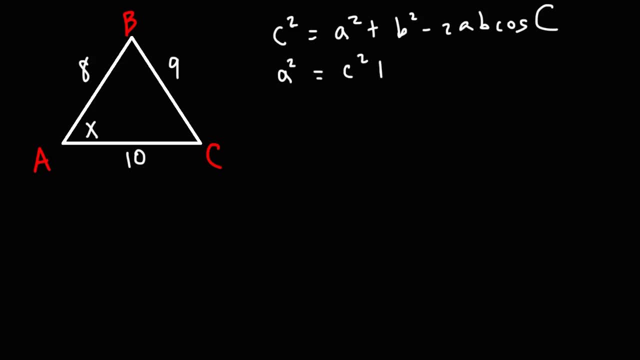 Another version of this equation, another variant is A squared is equal to C squared plus B squared minus 2B times C, or C times B, times cosine of angle A. 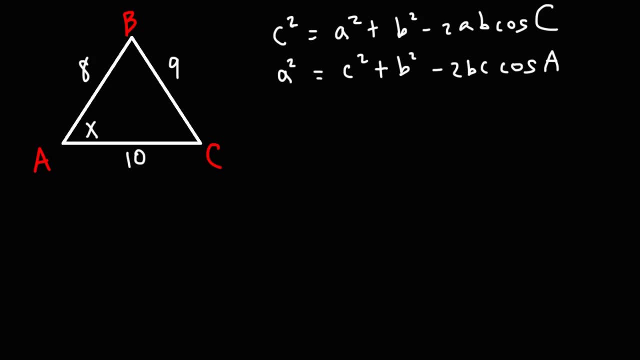 So that's another variant of the law of cosines. But what we need to do is get angle A by itself. 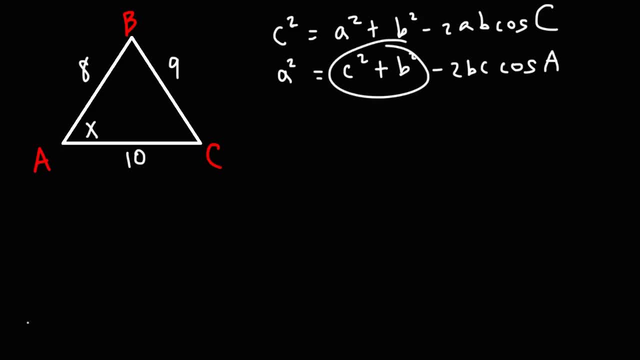 So I'm going to take these two terms and move it to the other side. And so I'm going to have A squared minus C squared minus B squared, and then I'm going to divide it by negative 2BC, that's going to equal cosine of angle A. 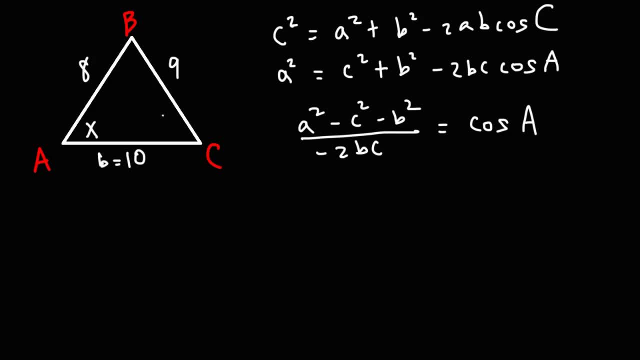 So in this example, we know that B is 10, because that's across angle B. 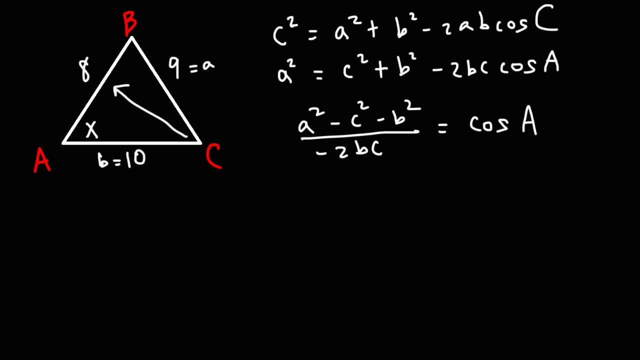 The lowercase A is 9, and the cross angle C is the lowercase C. So we can say that cosine of angle A is equal to A squared, which is 9 squared, minus C squared minus B squared, divided by negative 2 times B times C. 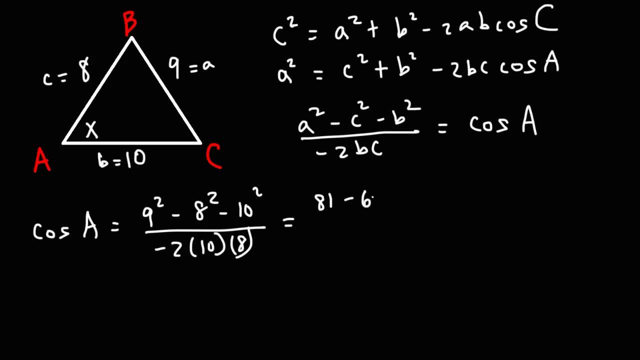 9 squared is 81, 8 squared is 64, 10 squared is 100. 10 times 8 is 80, times 2, that's 160. 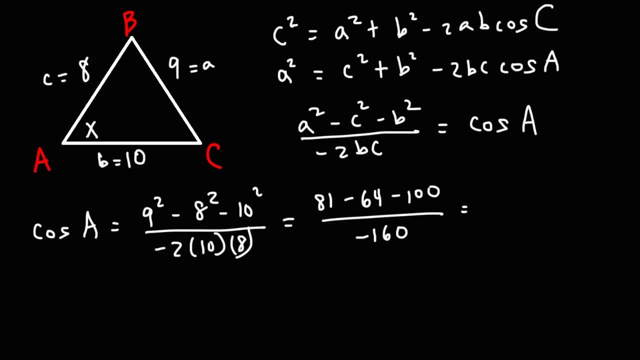 Now 81 minus 64, that's 17. 17 minus 100 is negative 83. So we have negative 83, divided by negative 160. 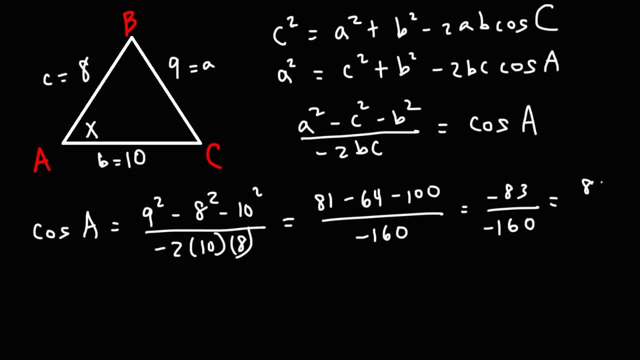 And you know what? We can just leave it like that. But the two negative signs will cancel. So what we have right now is that cosine of angle A is equal to 83 over 160. 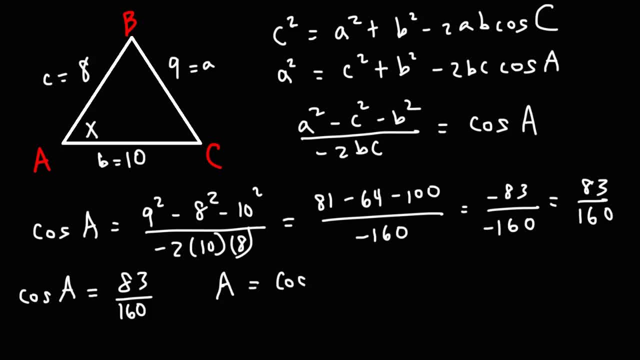 So therefore, angle A is the R cosine of 83 over 160. and if you plug that into your calculator you should get an angle of 58.75 degrees